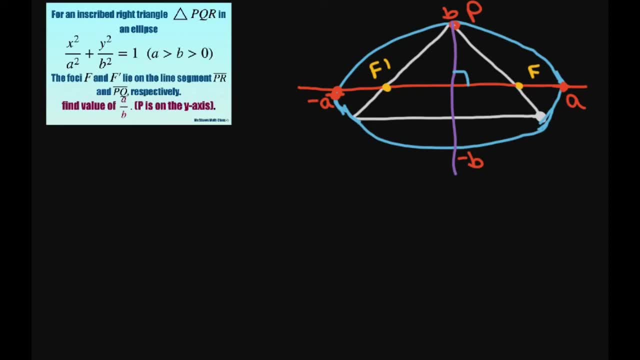 So here's my P. I did a little sketch here. My A is greater than B, so that means my A is bigger. That means it's the major axis. so we have negative A here and A. My B is smaller so it lies on the Y axis and also we have this point P. 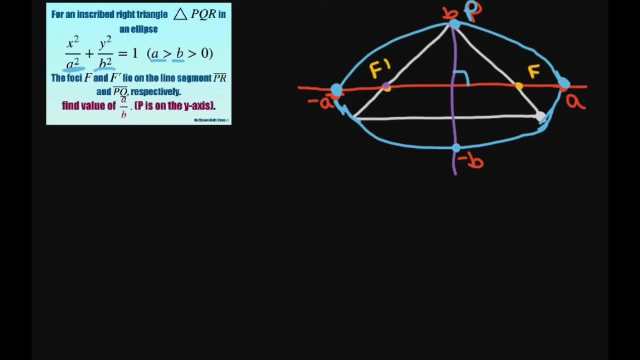 Also, it says the foci here lies on the line segment PR, so we'll call this R, and this is PQ, So we'll call this Q. So these foci lie on these line segments. Alright, so after we get that, I think I got everything. 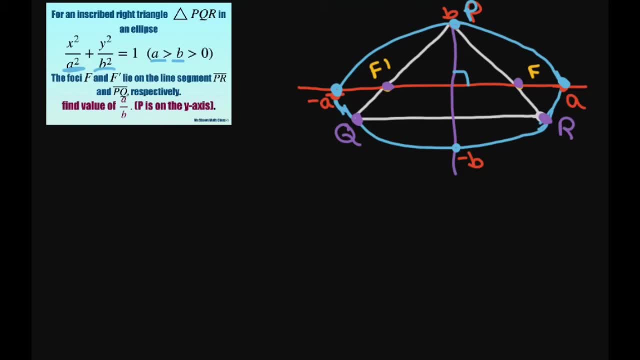 The measure. since P is on the Y axis, we have PF equals PF' and that equals A, So these two equal. P is on the Y axis and that means the distance between these two is 2A, But anyway, this just equals A, so we have that. 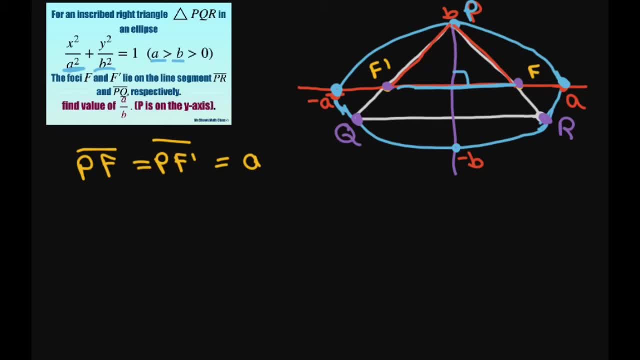 Alright, since we have the measure of angle, FPF', since these are equal, then this is 60 degrees. Alright, Therefore, my triangle, PFF' is equilateral, is equal angular. So that means this right here is going to be 60 degrees and this right here is going to be 60 degrees. 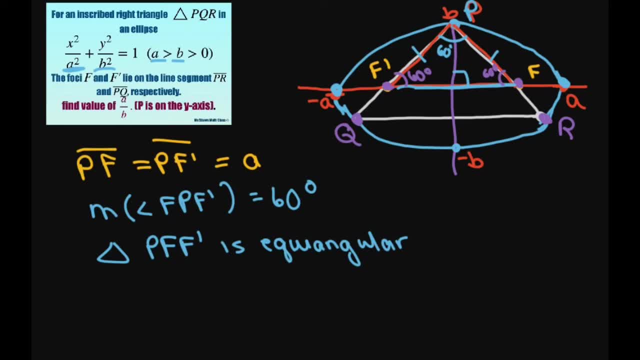 So all these side lengths are the same. Alright, Note that the height, The height of this triangle, the height is going to be PO and this length here is going to equal RB, right, Because we went up B and we went down B.